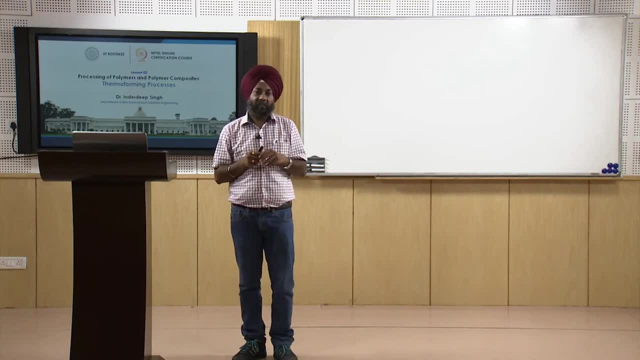 of the polymer so that it can flow freely and it can fill the mold cavity easily. So the first part is heating the polymer. The second part is molding or molding, So the molding or forming in which we give the desired shape to the polymer. So first step, first 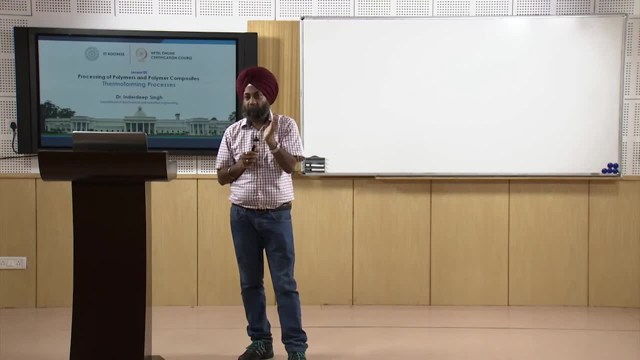 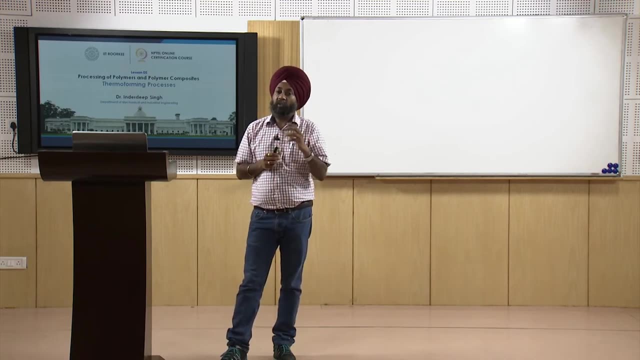 step is heat. second step is form f o r m. So we are going to deform, we are going to change the shape of the polymer, or we are going to give the desired shape to the polymer in the mold cavity. Now we can have different types of molds. 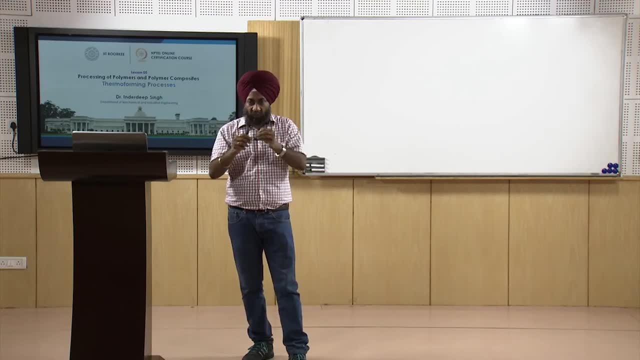 we can have different types of dies in which we will inject, we will force, we will allow the polymer to flow and then it will take the shape of the mold cavity. So again, coming on to the first two important points, point number one is heat. point number: 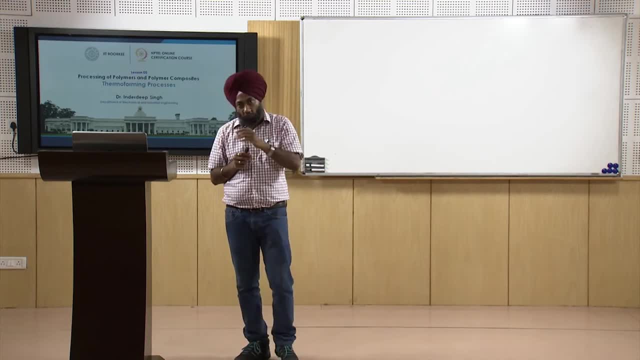 two is form. and point number three is cool. We will allow the mold to cool so that the polymer that we have injected, that we have forced, that we have allowed to flow in the mold cavity solidifies and takes the shape of the die, takes the shape of the mold. So 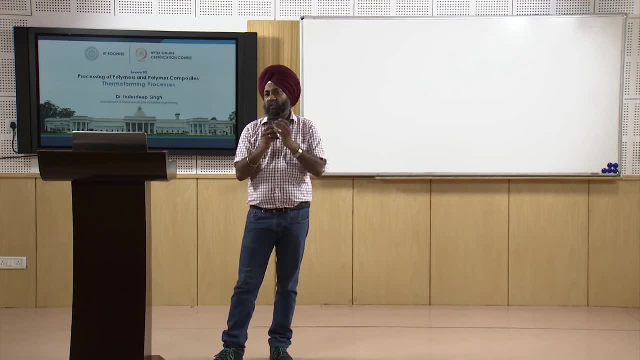 we can make heat. we can also allow the mold to cool so that the black membrane, red membrane and brown membrane and they become a little bit cool Now let us now go to the further part of the process itself. So that is when we need 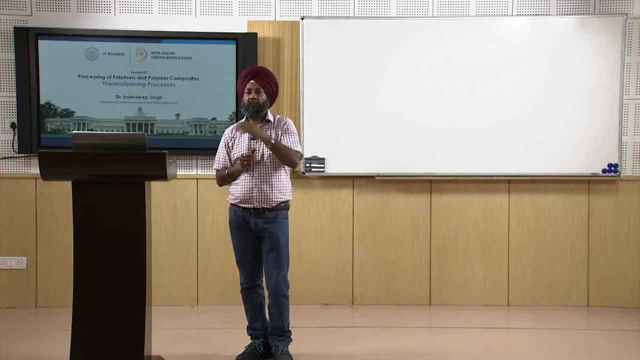 to semua exists all these processes, all the we get our final product. So all the processes that we are going to cover in our topic on processing of polymer, these three will be the main steps: jersey, which are not very thick, which are thin components, thin walled sections, and we will deform them. 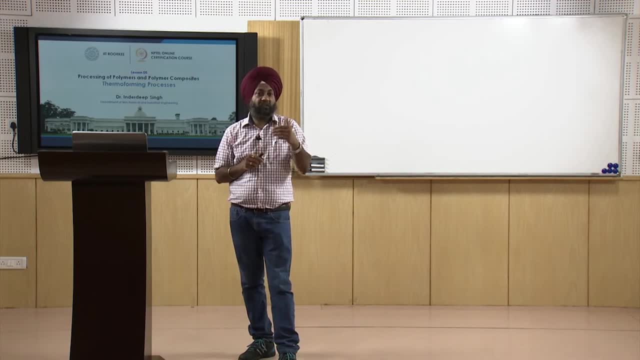 to give them the desired shape. so we will see what are the various applications of thermo forming process, what are the advantages of thermo forming process, what are the limitations of thermo forming process, as well as we will see that how thermo forming process is different, like what are the different types of thermo forming process. so let us first start our 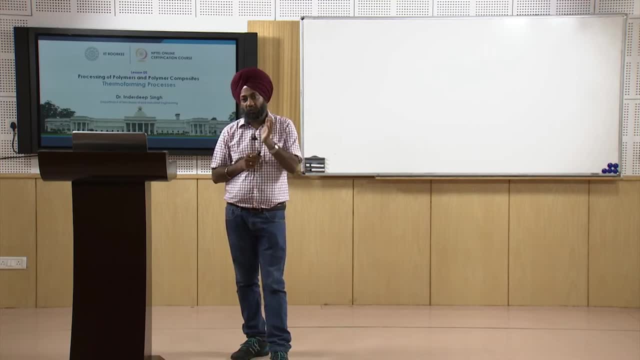 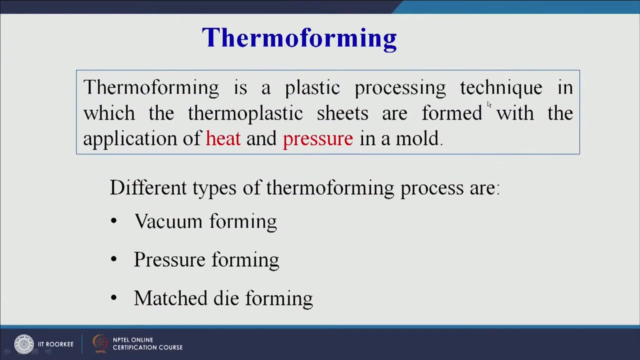 discussion with the types of thermo forming process, and later on we will come to the advantages, limitations as well as application areas for the thermo forming process. so let us start our discussion now. let us see what is thermo forming process. on your screen, you can see, thermo forming is a plastic processing technique, so it is a polymer processing technique in. 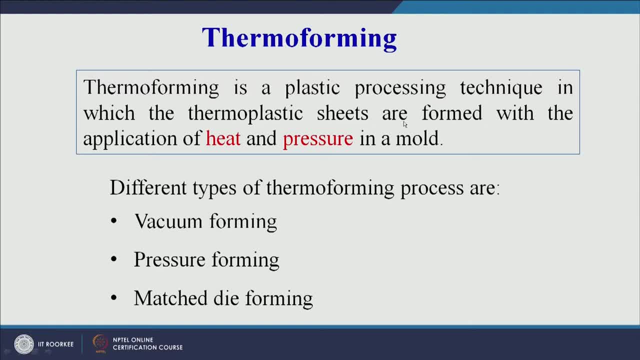 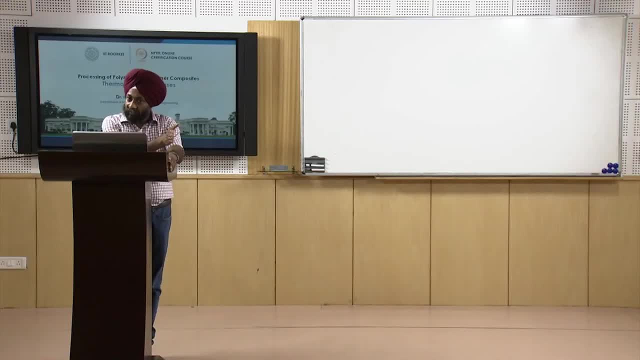 which the thermoplastic sheets are formed with the application of heat and pressure in a mould. so here, whatever i have discussed in the introductory part of today's session, heat is again coming into picture, mould is again coming into picture, and additional thing that we are supplying here is the pressure. 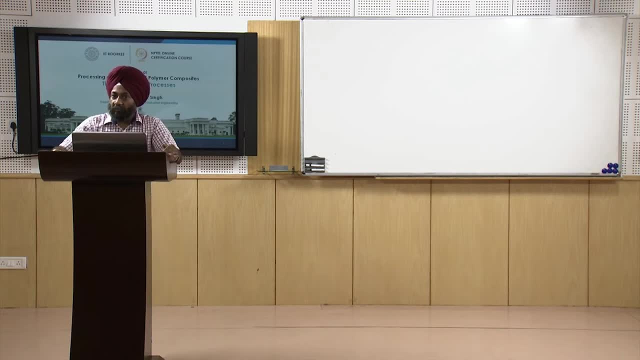 now, pressure can be in the form of mechanical pressure. it can be in the form of pneumatic or air pressure. it can be. pressure can be applied even with vacuum and, based on the method with by which we are applying the pressure, we classify the thermo forming processes into. 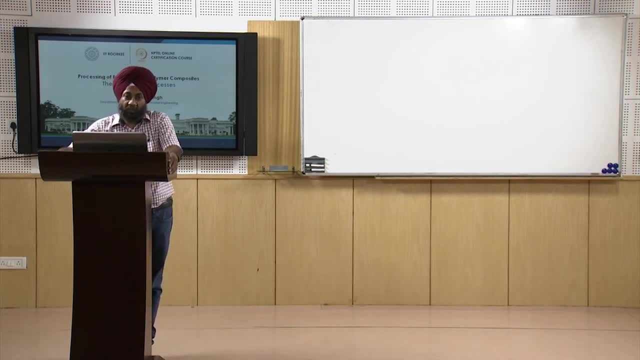 different types. we can have vacuum thermo forming, we can have pressure thermo forming, we can have matched die, which is a mechanical type of thermo forming process. so each one of these we will try to understand with the help of a specific schematic diagram. so first of all, we need to understand that this is used for thermoplastic sheets. so again i am. 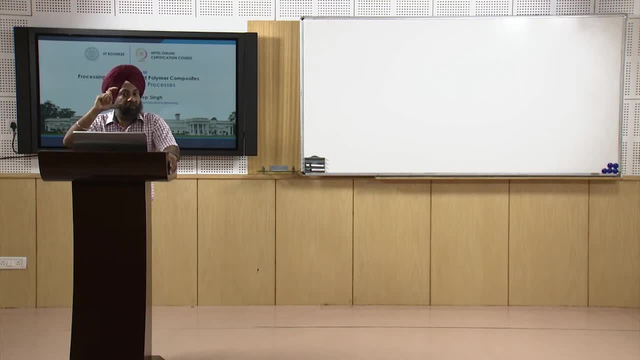 emphasizing that thermo forming process is a process which we are applying to different materials, yet we are using the process also here, what they call heat transportation process, so heat transportationgrade a plastic, we call it heat transport process. so heat transport process is basically equal to the number of gets, to essentially say l, the temperature. 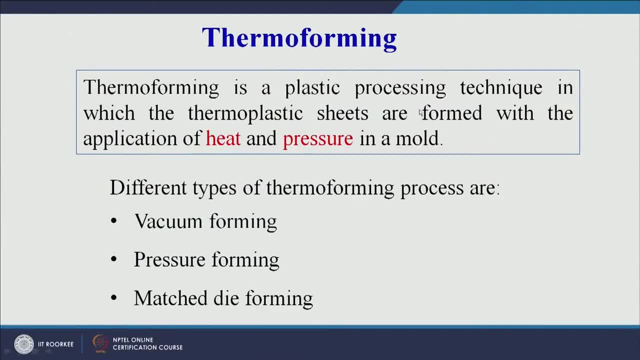 again heat into to reduce in. we are going to be using is carriers as transfer to cameras. we are giving probability O, which is V2 equal to 1, and V2, which is V1 equal to 0, and V3� is equal to Vk, and you just apply the temperature, that we shall see an M p, which is and method. 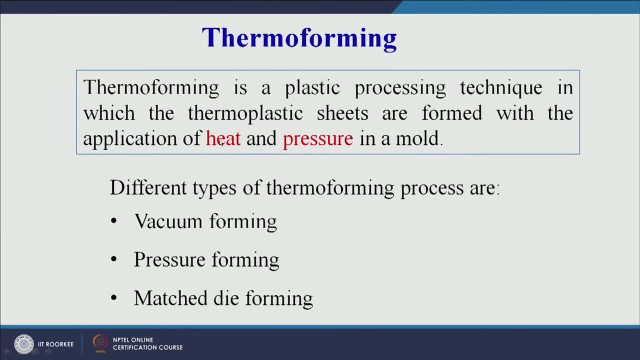 introduced in this material isαassen the time a procedure which is used to define the structure, isapplied for that, and then you can use it in a different way. suppose, leave it to form aоль-лен and theanna. sheets are formed with the application of heat and pressure in a mold. another point: 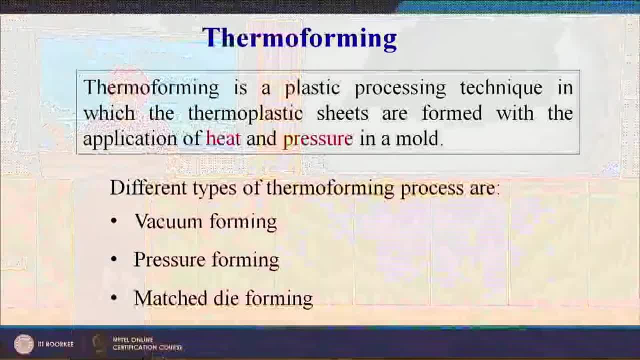 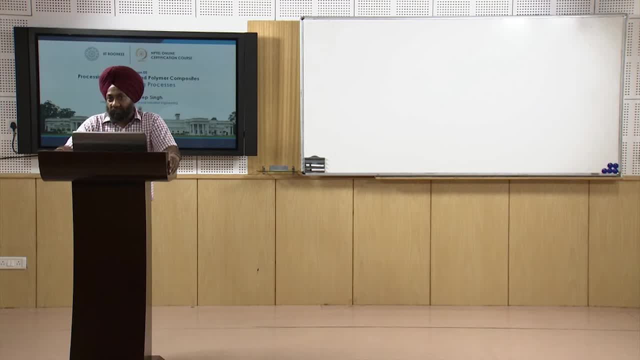 that you should remember here is that this is thermo plastic sheets. so, if you remember, we have classified the polymers, or plastics, into two broad categories, that is, thermosets and thermoplastics. so thermo forming process is specifically ah applicable to thermoplastics, whereas in some special cases may be, the process may be modified slightly to be suitable. 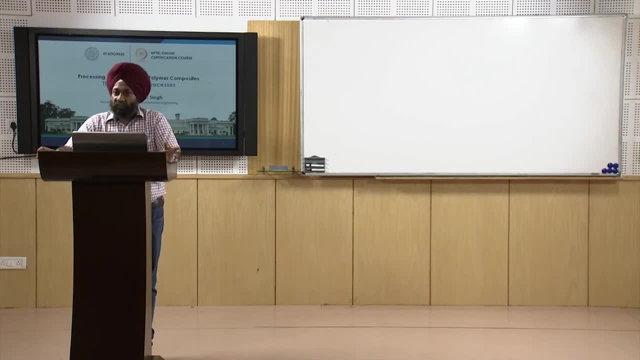 for thermosets also, but majority of the cases thermoplastic will be the raw material for the thermo forming process. now, different types of thermo forming process, as you can see on your screen, is vacuum forming, pressure forming and matched die forming. so we will try to. 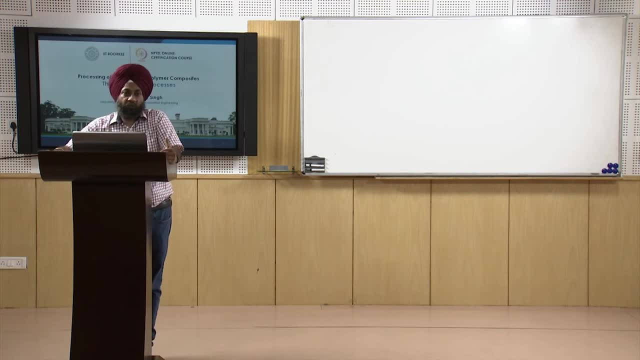 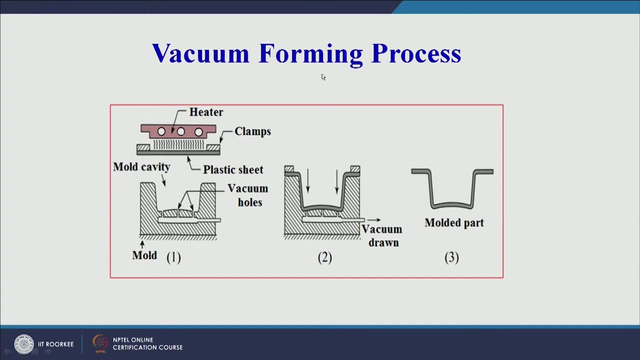 understand the basic working principle of each one of these classification of the thermo forming process. to start with, on your screen you can see we have a basic diagram of a vacuum forming process. in vacuum forming process, let me first read out what is there on your screen. there is a heating arrangement, there are clamps. there is a raw material- thermoplastic. 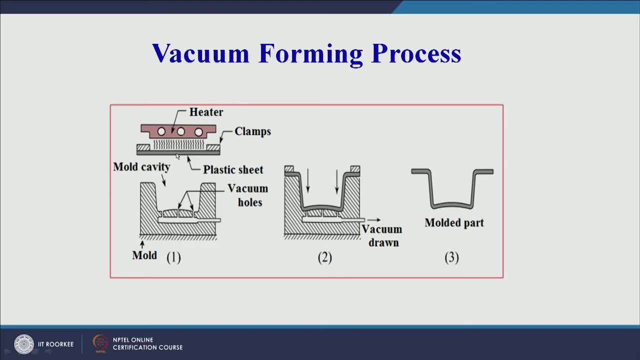 sheet, this gray color sheet, on your screen, you can follow the cursor. this is the raw material which we want to define. so here you can see. once this sheet is heated, the mold is closed, the this particular clamps come here and the sheet occupies this position on your screen you can see. and finally, when we apply, 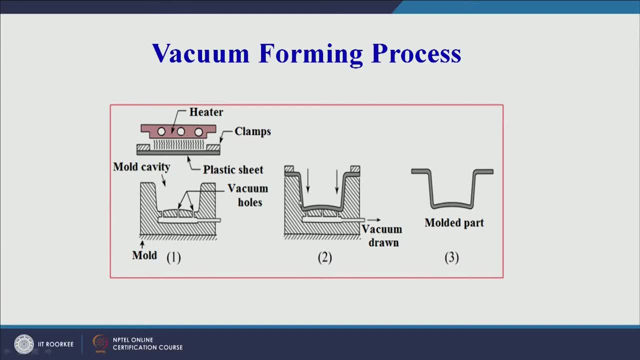 the vacuum. through this vacuum holes, the sheet is pulled down to confirm to the shape of the mold. now, whatever will be the shape of mold, the sheet will confirm to the shape of the mold. why? because of the pull exercised by the vacuum in the bottom, we have a vacuum. 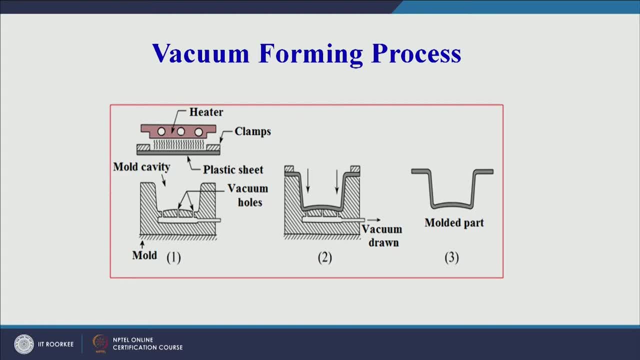 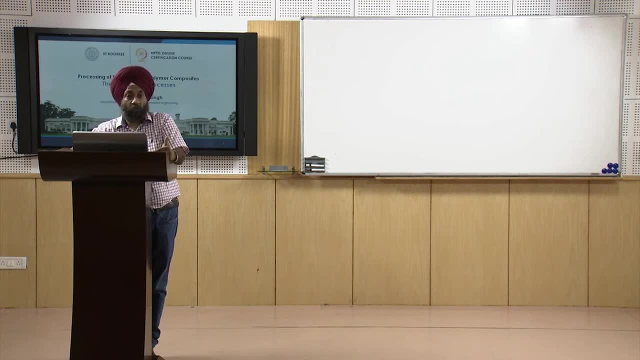 should vacuum will pull the sheet down and it will confirm to form, as there is a vacuum, conform to the shape of the mold. so i think it is a very simple process. now we are not going to go into the details that how much vacuum is required. what can be the typical? 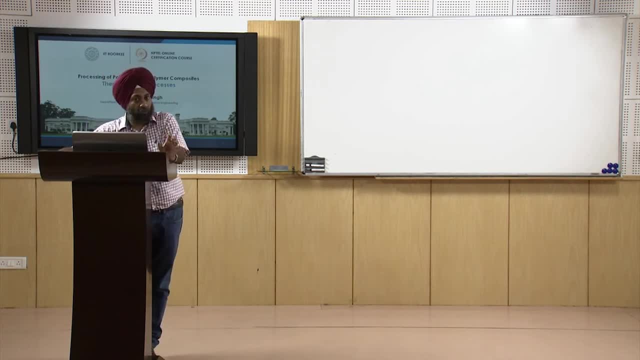 thickness of the sheet. we are currently focusing on the basic working principle of the vacuum forming process. we should know that this is this process is used for thin sheets. the raw material of the sheets is thermoplastic and we have to apply a vacuum so that the sheet 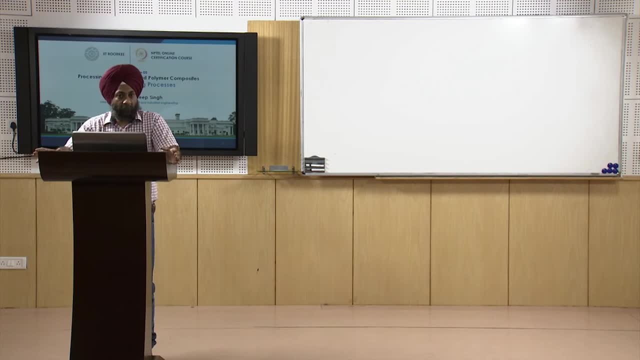 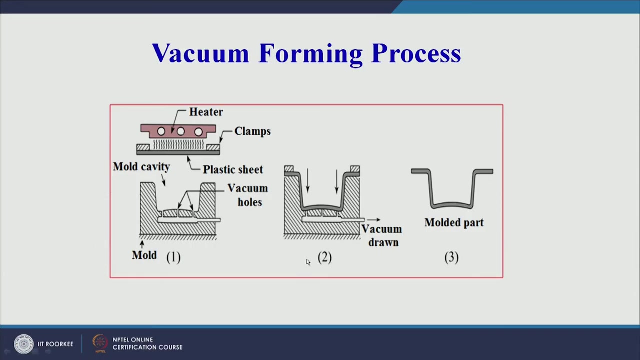 conforms to the shape of the mold. if that much we can remember, we will never forget the vacuum thermo forming process or the vacuum forming process that falls under the category of thermo forming. now on your screen you can see, as in the part two or the step two of 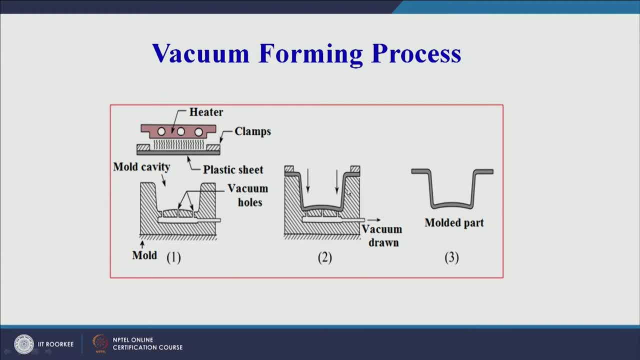 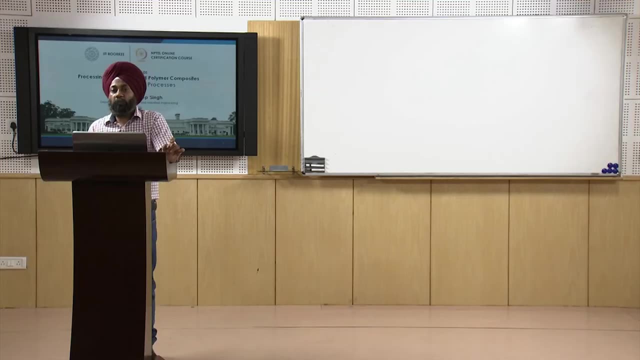 the process. the sheet is conforming to the shape of the mold after the vacuum has been drawn out, or the after the vacuum has been applied, and this is the final molded part that we can produce using the vacuum forming process. now, whatever i have explained, let us try to systematize. 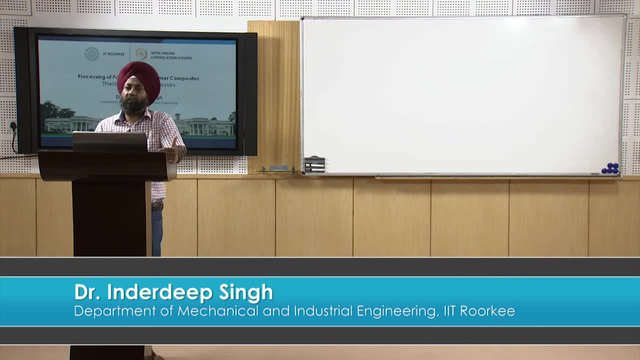 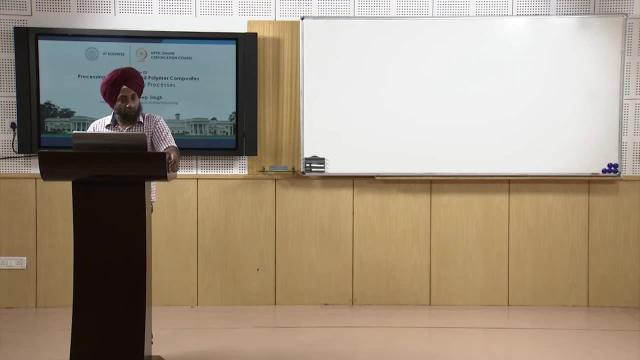 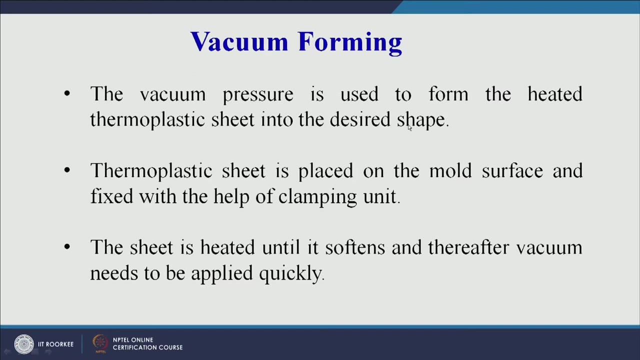 it. let us try to study it step by step so that you remember the basic working principle of the vacuum forming process. on your screen you can have a look at the various stages, steps or the basic working principle of the vacuum forming process. the vacuum pressure is used to form the heated thermoplastic sheet into the desired shape. 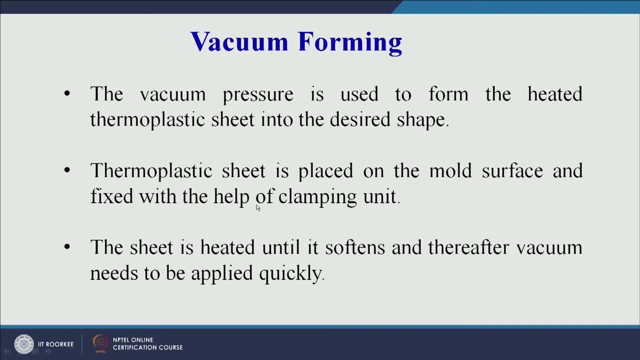 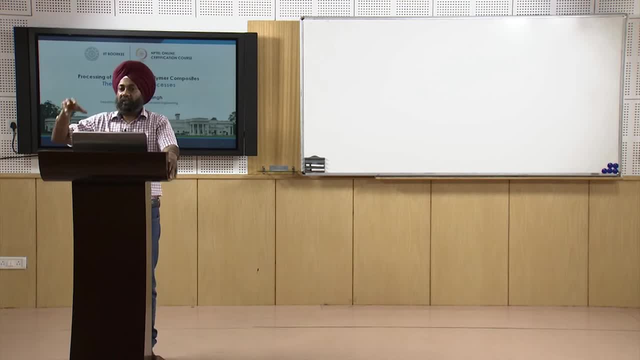 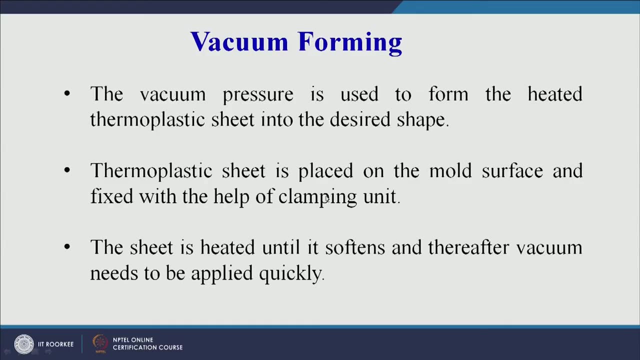 cold poking, hot torching fireporte. so now another Paleo пятnation borrowed idea i will show you. let us try. one is that you know first theaw manner in which you can do a lap, perform in any situation. you have to have a certain temperature or temperature, your whole body and your whole body temperature. 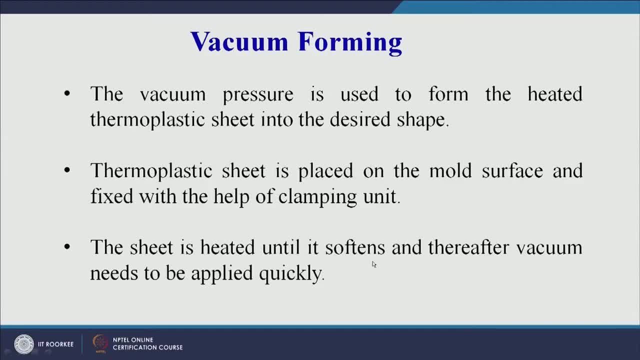 which depends from the temperature of your body, temperature coming from temperature of your Algiansueelo, or체 and nori temperature. according to the temperature, if we stupidly compute the magnetic толsうん and hot ٩ sru Char myself also mono sapon, also known as. 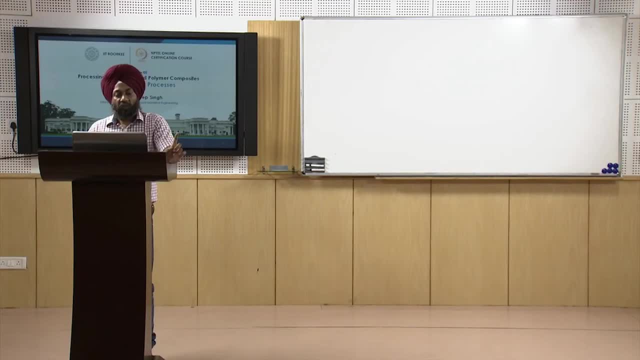 therこと force that we have to supply. so the sheet will be heated until it softens. why do we need to soften the sheet? because we need to deform the sheet in the next stage. if we soften the sheet, it will be easy for us to deform it as per our requirement. that is given in 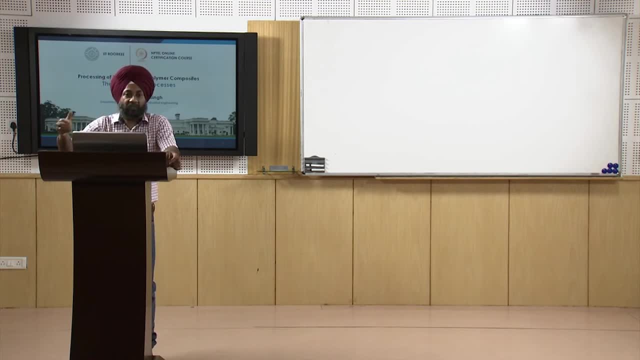 the design of the mould. our requirement is already present in the form of the mould, because the mould is the exact replica of the product that we want to make. so as per our requirement means the sheet. if the sheet is soft, it will deform easily into the mould. it will conform. 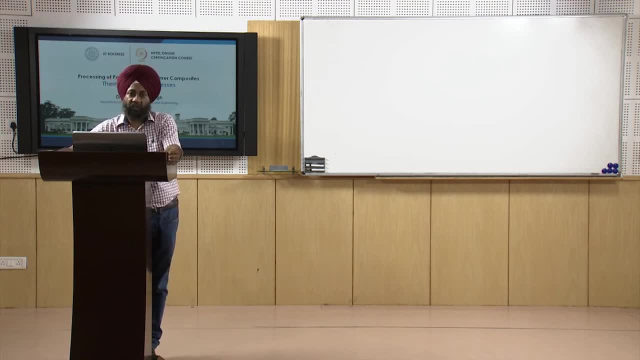 to the mould shape. that is our requirement, that is the product that we want to make. so the sheet is heated until it softens, and thereafter first we have to ensure that the sheet has to soften. then only we will apply the vacuum. therefore the requirement of vacuum will also. 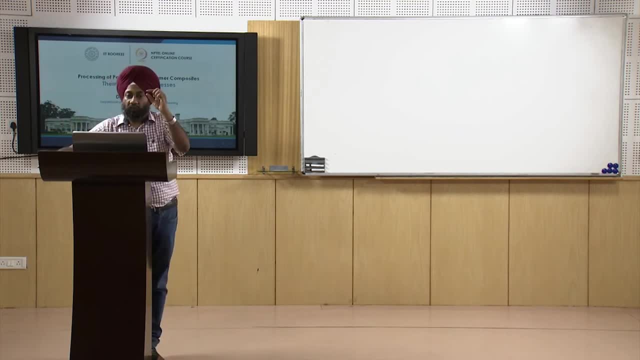 be depend will also be dependent depending on the thickness of the sheet. it will also depend upon the state of the sheet. if it is not soft, suppose it is very hard, so the vacuum has to be applied accordingly. so first, what we will do, we will soften the sheet so that the requirement of vacuum is 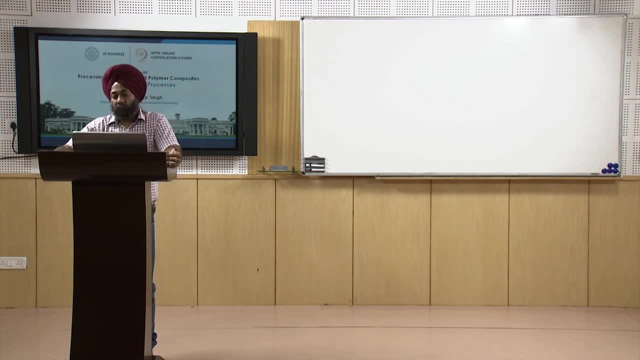 also optimized. so the sheet is heated until it softens and thereafter vacuum needs to be applied quickly. so as the sheet is soft, we will apply the vacuum. the sheet will be pulled down as per the shape of the mould, So that we have already seen with the help of diagram, a search tank is used to quickly. 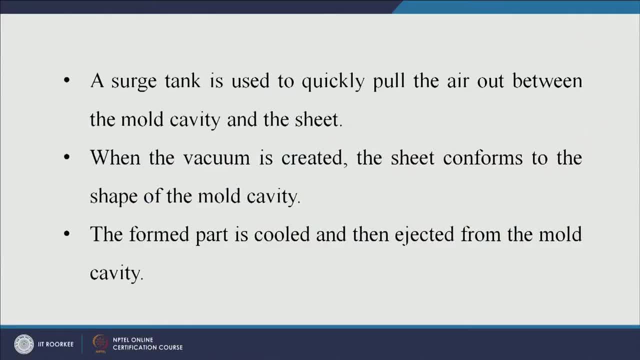 pull the air out between the mould cavity and the sheet. that is a method of applying the vacuum, the. when the vacuum is created, the sheet conforms to the shape of the mould cavity that i have already explained. the formed part is cooled and then ejected from the mould. 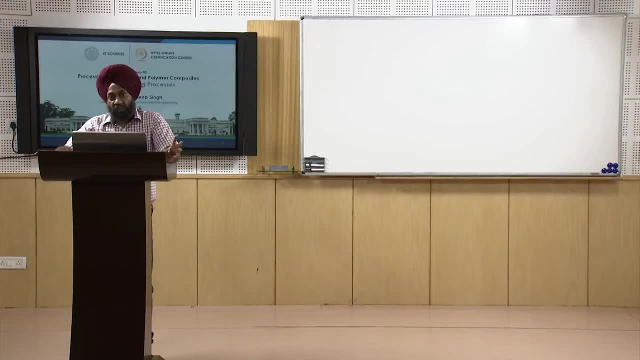 cavity. so the third step, now cooling. so three step process: heating, forming and cooling. so finally, when, once the part has cooled, or once the mold has cooled, the part or thermo formed part is taken out and that is our final product. at the later stage we may require some kind 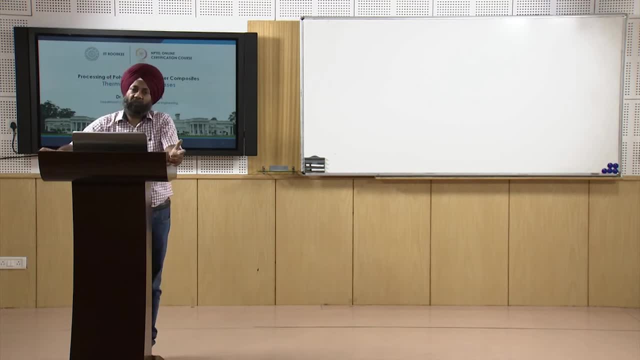 of trimming. we may require some kind of finishing before we can use that part, but we will get our final product as a as a final outcome of this vacuum thermo forming process. so this is a first classification of thermo forming process which is based on vacuum, the pressure. 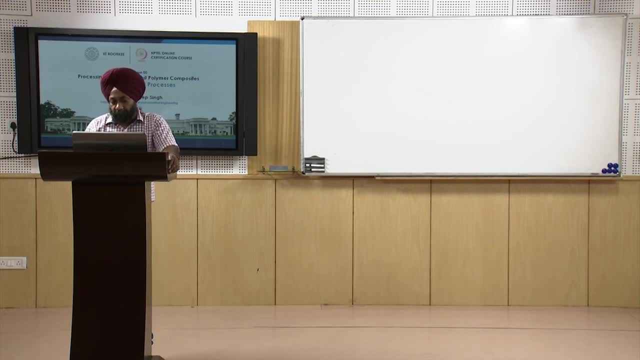 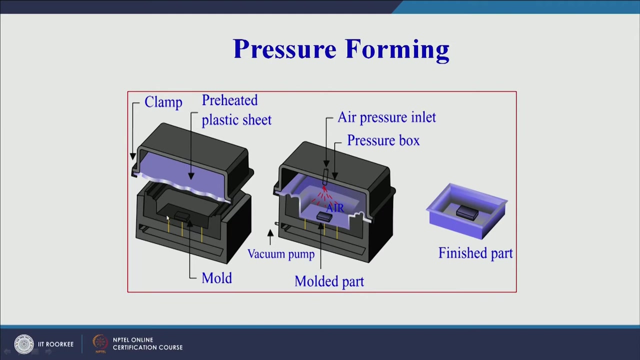 is applied in terms of vacuum. the second process that we want to cover today is pressure forming. so here again on your screen, we see a diagram. in the diagram we can see there is a clamp. the clamp will fix the two parts of the mold, so there is a upper mold part. 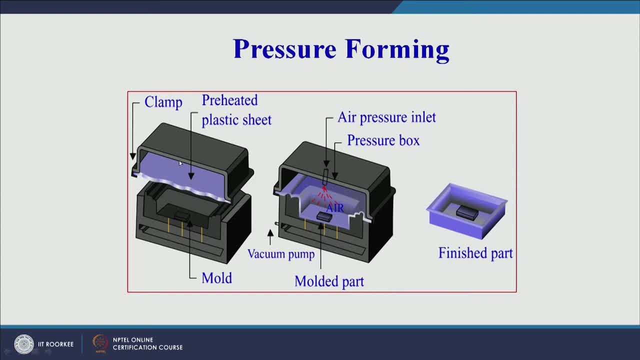 and there is a lower mold part. on the screen you can see this sky blue color sheet is the preheater part and this is the coolant temperature and the second process we want to cover today: heated plastic sheet. so in this case, what we will do, we will have a preheated plastic. 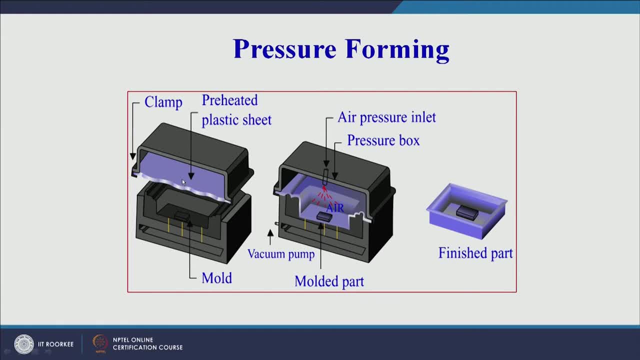 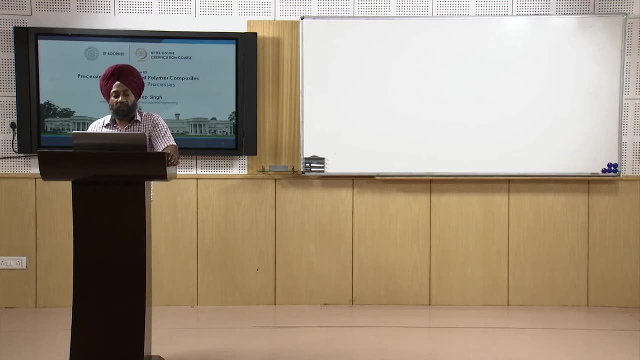 sheet. in previous case, if you remember, in case of ah, vacuum thermo forming, we were having a heating arrangement, so the sheet was being heated in the setup itself. but here we need to have a preheated sheet. so we have a preheated plastic sheet and we have two part mold that 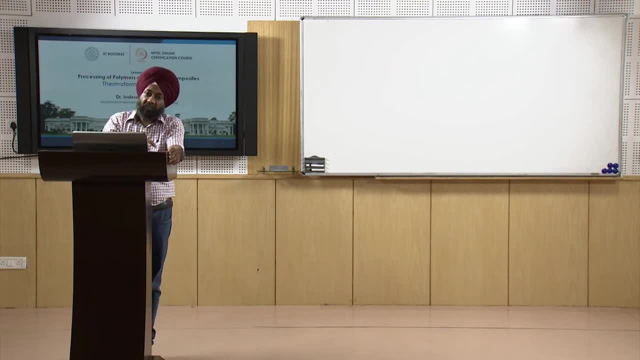 we will close and apply the pressure on this preheated sheet so that it conforms to the shape of the mold and we get our final product. so here you can see the two part mold. then there is a clamping unit which will clamp the two parts of the mold together and then 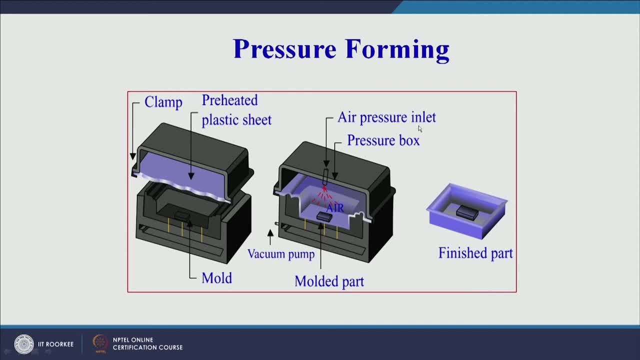 the air pressure inlet is there through which we will supply the pressurized air to apply pressure on this sheet so that the sheet conforms to the shape of the mold. so you can see this is the molded part here. the sectioned view is here shown. here we see the final part, how the final part or the final product would look like. 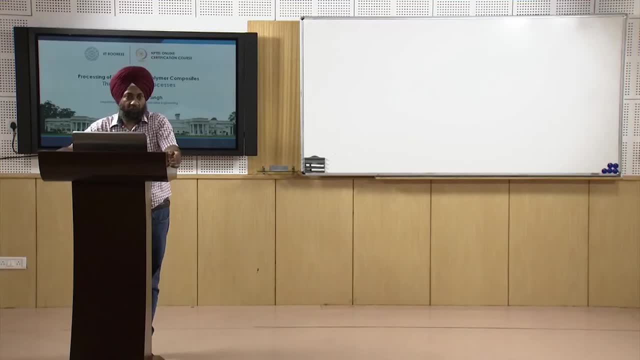 so the difference between the two- that is, a vacuum forming process as well as the pressure forming process- is the mechanism of applying the pressure or the mechanism of forcing the sheet against the mold. so in case of vacuum, we apply vacuum so that the sheet is pulled as per the mold cavity or as per the design of the mold cavity. 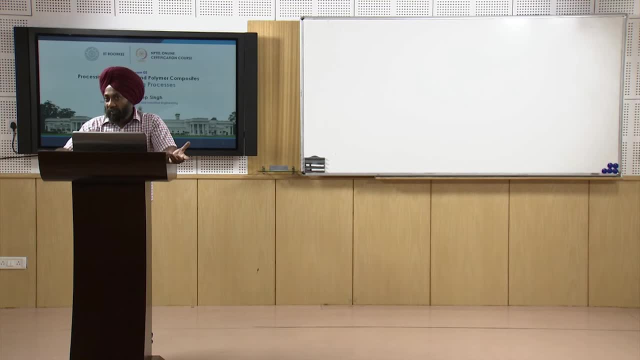 so we will form the sheet based on vacuum. in case of pressure forming, we are pushing the sheet. if you see the diagram, this is the sheet. this is a sheet. we are pushing it down how, with the application of air pressure? so we will. we are applying air pressure to force the 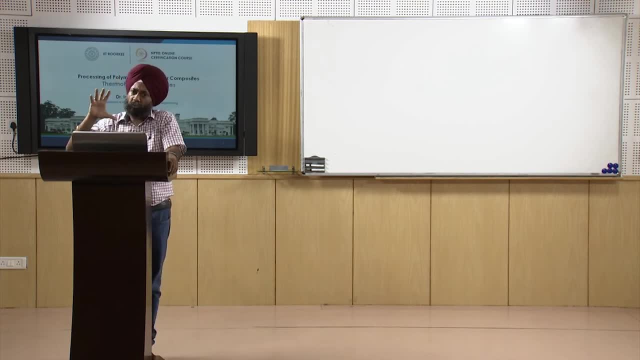 hot or the heated sheet or the preheated sheet against the walls of the mold, so that the sheet conforms to the walls of the mold and takes the shape of the mold. that is the exact replica of our final product. so mold is designed as per the requirement, as per our final product. 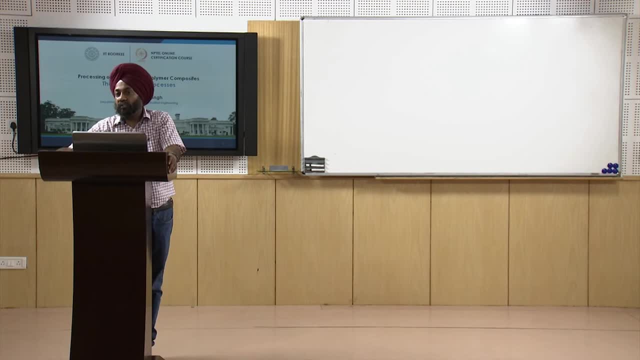 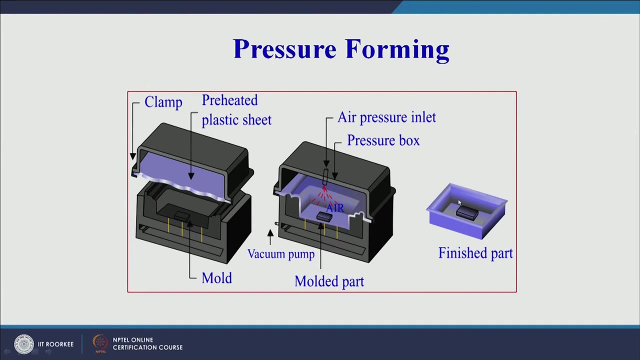 so we are forcing the sheet with the help of air pressure against the walls of the mold so that we get our desired product. so here you can see the final product, or the finished product is shown on your screen. this is the final product, so this is the basic working. 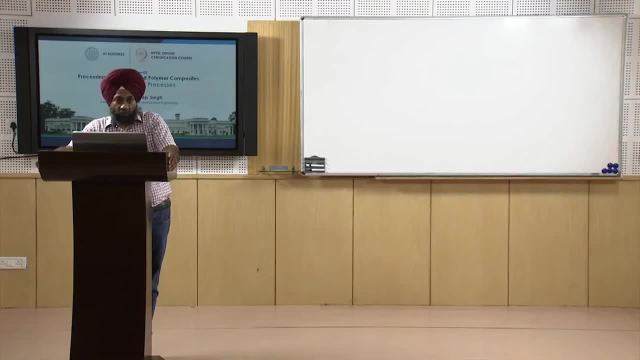 principle of the pressure forming process. now here, if you see, if we have to control the process, we need to see that what can be the thickness of the sheet, what, what is the amount of pressure that is required and for how long the pressure is required. how much time is the sheet will take? 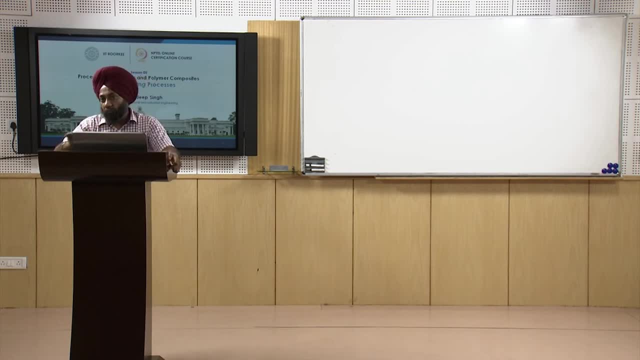 to conform to the wall or the conform to the shape of the mold. so all are the. all these are control parameters that we need to take into account when we are working with the pressure forming process. we will get different types of defect. we may get non uniform thickness. 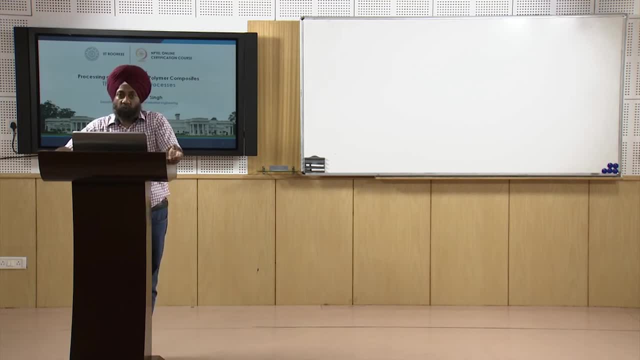 of the sheet once the product is ready. that may be because of non uniform thickness of the sheet will be affected by the application of pressure on the sheet. so there can be number of defects that can arise due to non, non optimal or due to wrong selection of the process parameter, such as the application of air, air application of air pressure, the 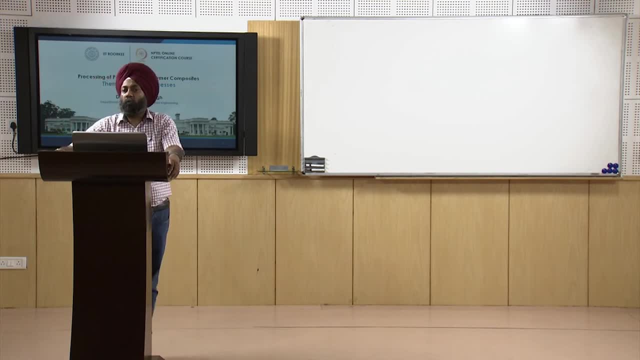 holding time, the, that is, the cooling time, then the time for which you are applying the pressure. all these are important parameters that have to be taken into account in order screen. so we have seen two types of thermo forming processes. one is vacuum forming, another one is pressure forming. now let us try to understand the third type of process that 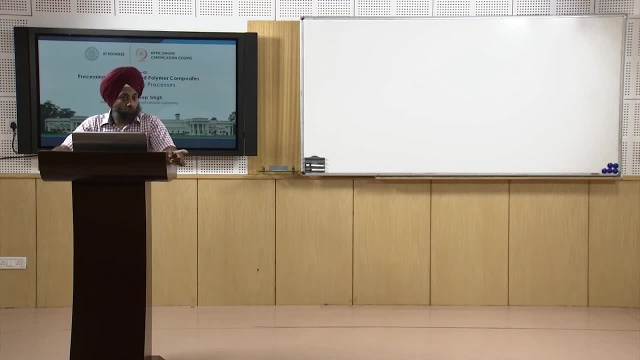 is the mechanical forming. but prior to going to the mechanical forming process, let us first just revise what we have covered in pressure forming. i have tried to explain with the help of a diagram, but whatever i have said, we have summarized it in six or seven points. so i 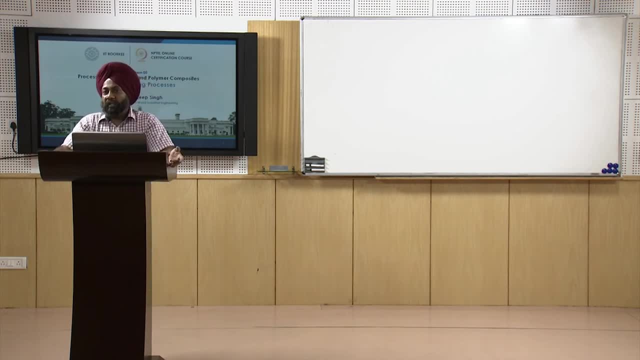 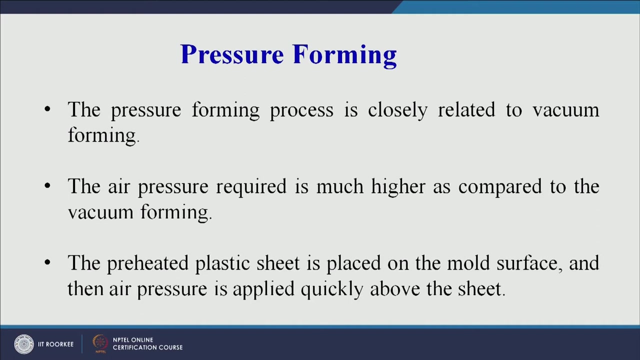 will quickly read this point and then we will move on to the mechanical forming process. that falls under the category of thermo forming processes. so the in case of pressure forming, the pressure forming process is closely related to vacuum forming. i have already explained the difference between the two. the air pressure required. 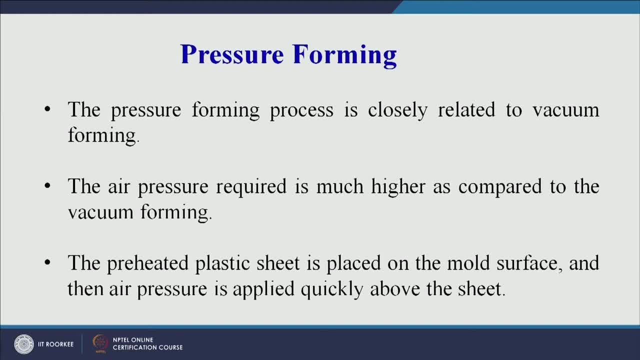 is much higher as compared to the vacuum forming. the preheated plastic sheet is placed on the mould surface and then the air pressure is applied quickly above the sheet. the high pressure pressure is developed in between the softened sheet and the pressure box due to high pressure. 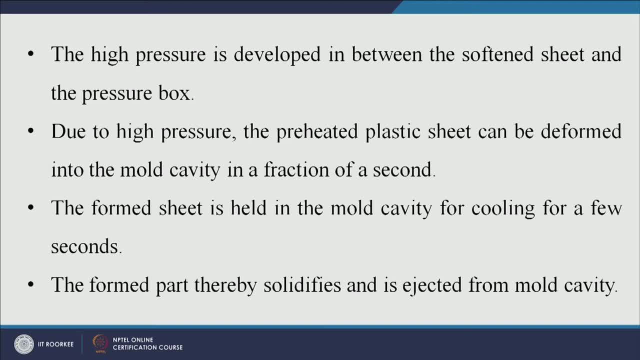 the preheated plastic sheet can be deformed into the mold cavity in a fraction of a second, so it doesnt take much time. the formed sheet is held in the mold cavity for cooling for a few seconds. the formed part thereby solidified, gets solidified or solidifies and is ejected. 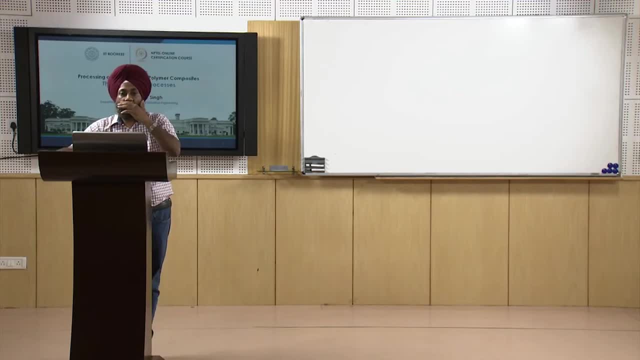 from the mold cavity. so these are the important steps, or the sequence of operations that are carried or carried out, in order to successfully deform a preheated plastic sheet into a tangible product. so we have seen two broad variants of the thermo forming process. let us now see the third variant of a thermo, of the thermo forming process, that is, the 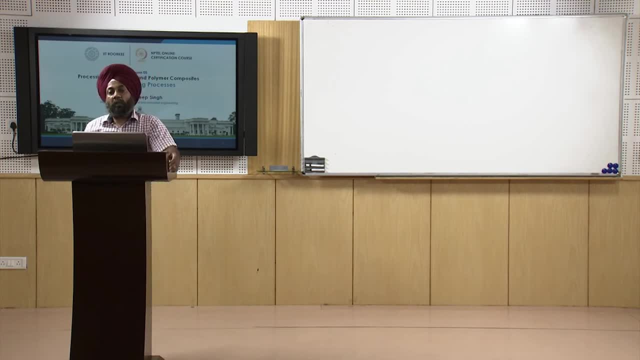 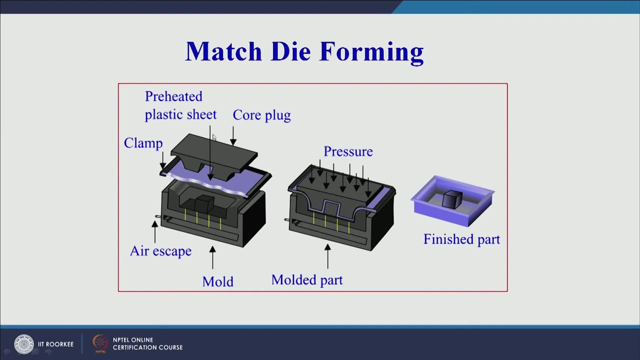 mashed die forming. in mashed die forming process you can see- let us first see the diagram properly- we have a preheated plastic sheet. so in this case also we will have a preheated plastic sheet. you can see the sheet here again, the sky blue color sheet. then there is a clamping unit, there is a core plug. now, core plug is different. 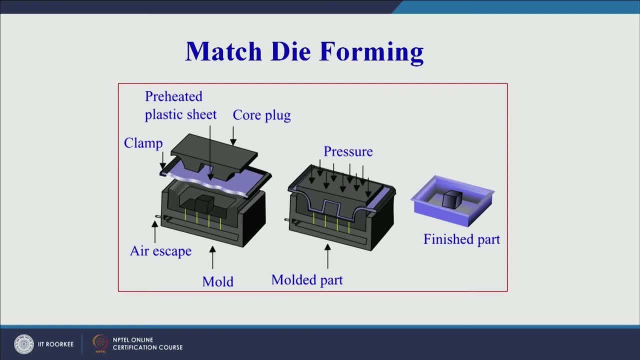 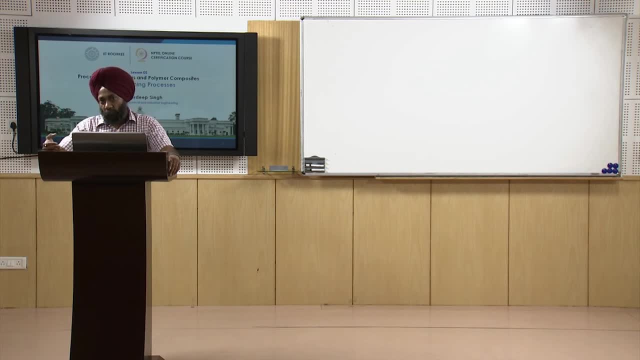 from the first two processes. in case of vacuum forming, we had a heating arrangement on top of the sheet. in case of ah pressure forming, we had a pressure box on top of the sheet. now, in case of match die forming, we have a core plug on top of the sheet. now, this core 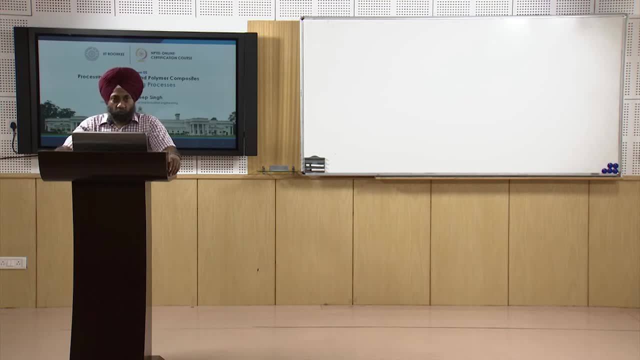 plug is used to apply mechanical pressure on the sheet so that the sheet deforms as per the mold cavity. so here we have core plug here, preheated plastic sheet clamping unit. then there is air escape because once you are forcing the sheet against the mold wall. 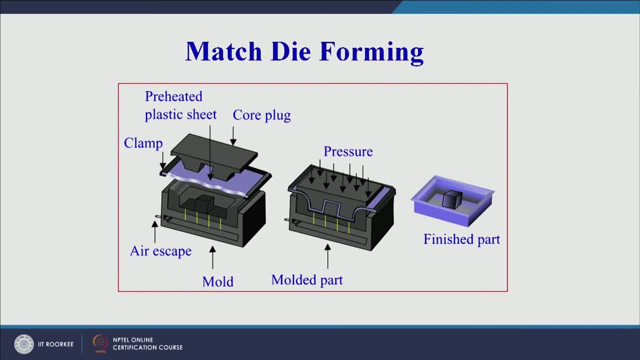 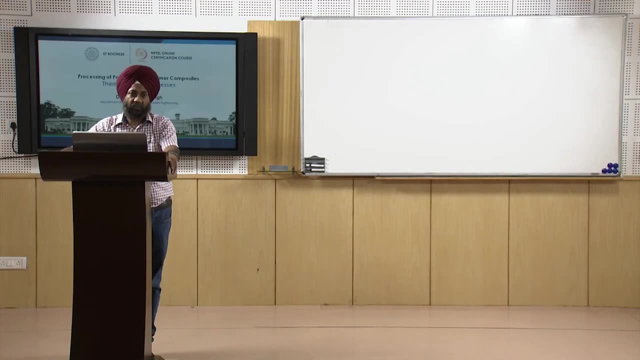 the air has to be released, whatever air is present inside the mold, and then we have a mold which is the final shape that we want to produce. so here we can see, the mechanical pressure is applied. the core plug is used to push The sheet or the thermoplastic sheet against the walls of the mold so that the sheet conforms. 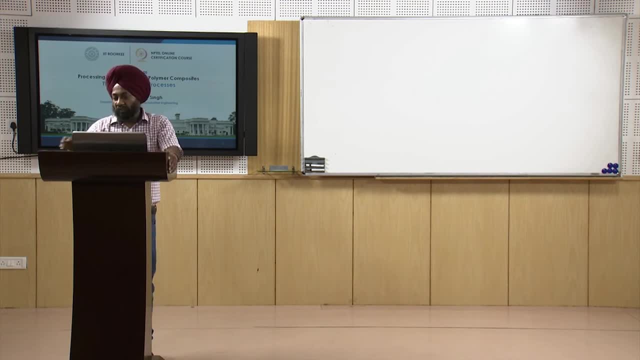 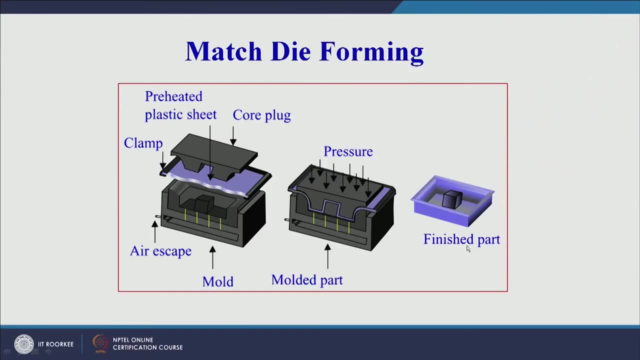 to the shape of the mold cavity and we get our final product. so here you can see, this is the final product that has been formed. that is a finished part. so this is the closed mold or core core plug, as come down, and the and the gap between the core plug and the. 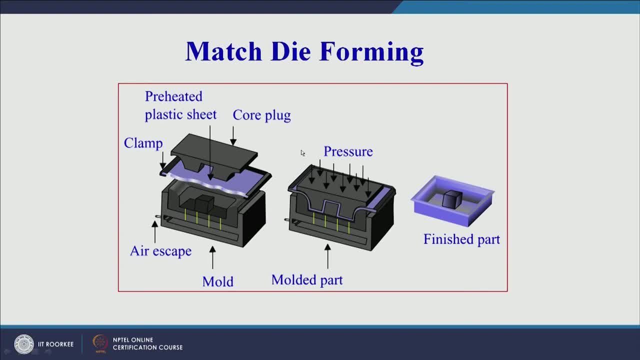 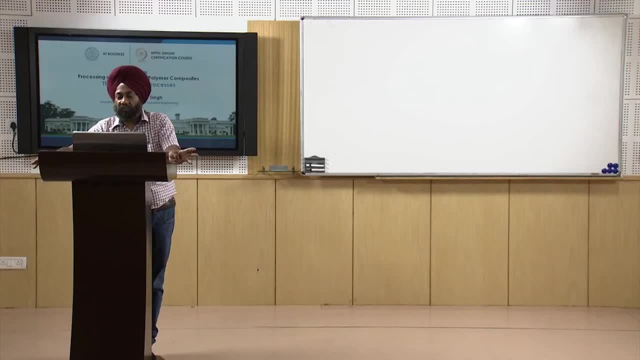 mold is filled by the thermoplastic sheet. so here we can see the three types of the types of processes, and the basic principle remains the same, the important three steps. remains the same, that first we have to heat, whether it can be within the setup also, or 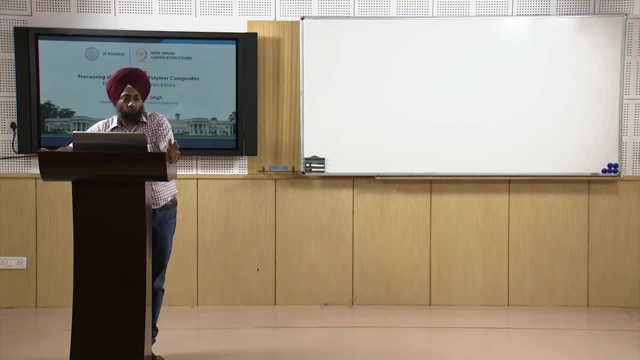 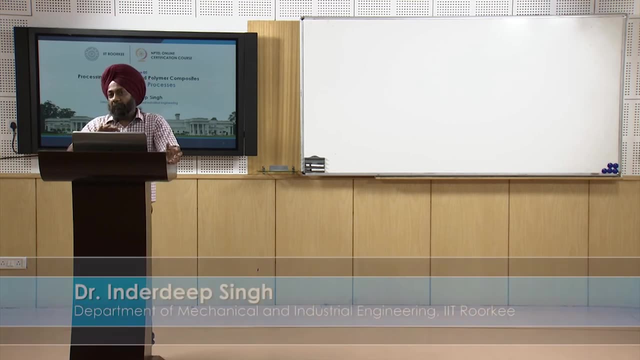 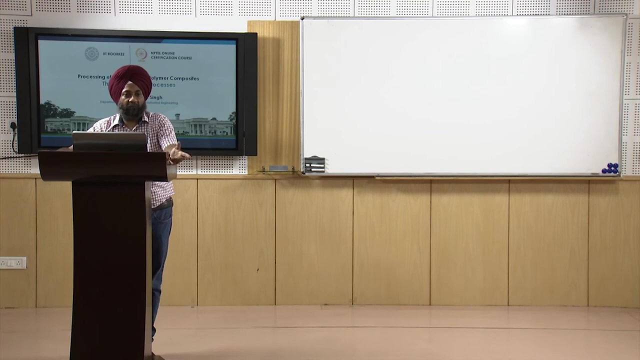 we can have a preheated sheet. so first thing is we have to heat the sheet. second is we have to deform it, apply the pressure. the deformation is happening or the forming of the thermoplastic sheet is happening because of the pressure. in this case. now pressure can be applied by 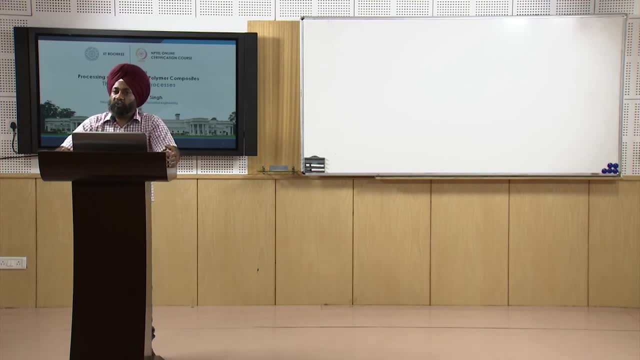 different means, as we have seen. and finally, we will allow the sheet to cool so that finally our final product is ready. so the three major steps of antipolymer processing technique are again being repeated in case of thermo forming process also. so the classifications we have seen. now let us go through the advantages, limitations, application, areas of the thermo. 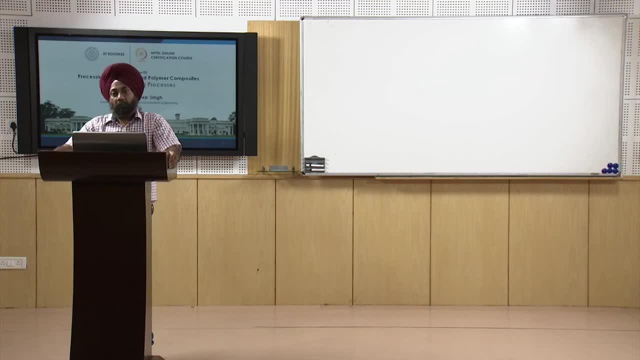 forming process. before going to the thermo application areas, let us first quickly have a look at the various steps involved in the match die forming process. i have tried to explain the match die forming process with the help of a diagram. now let us see that. how, or what are the various steps involved in the matched die type of thermo? 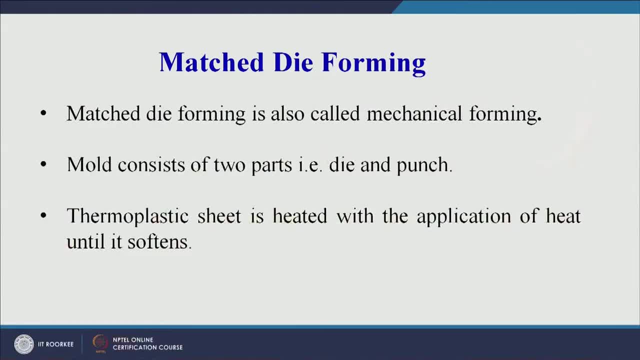 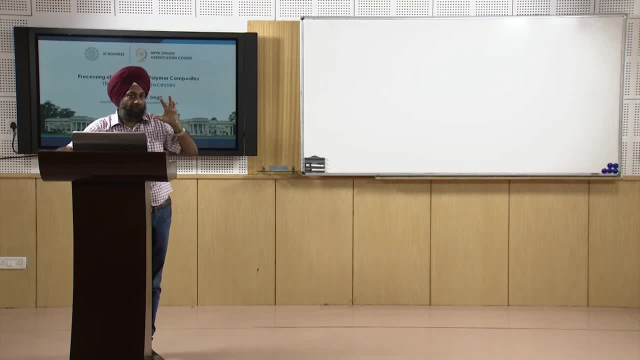 forming process. match die, thermo forming or match die forming is also called mechanical forming. now why mechanical? because in pressure forming, the pressure is applied by a jet of air. in vacuum forming, the pressure is applied by a vacuum. in case of matched die forming or mechanical forming, the pressure is applied mechanically by the core plug on the thermoplastic sheet mold. 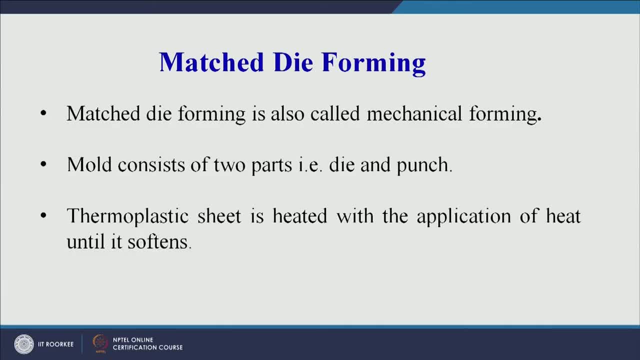 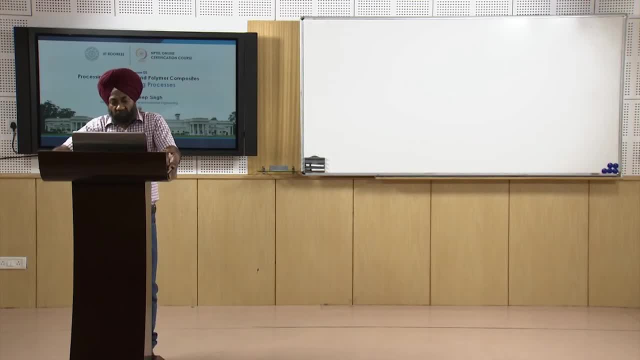 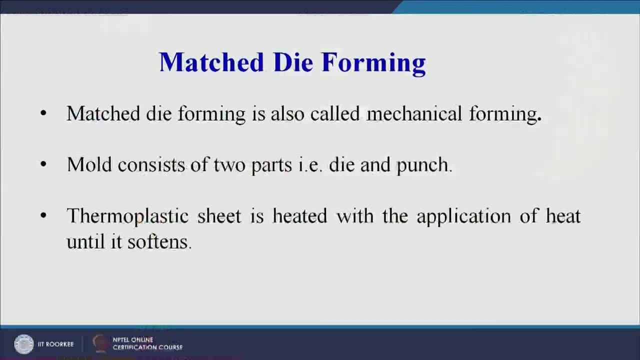 consists of two parts: die and punch. so the core plug in this case acts as a punch and it forces the sheet against the mold, against the mold walls. thermoplastic sheet is heated with the application of heat until it softens, as in the diagram it was given. heat is a prerequisite. 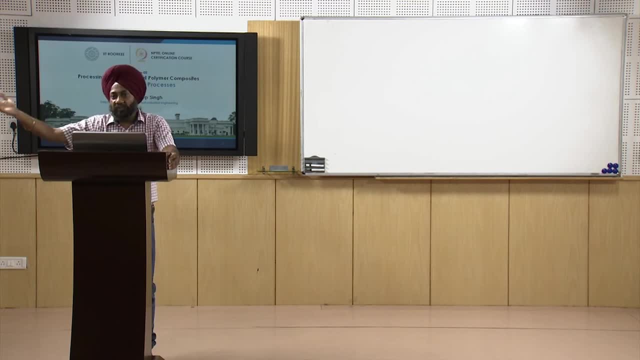 thermoforming and the sheet can be preheated in a different setup and then can be brought to the molding setup or within the setup. also we can have a heating arrangement where we can heat the sheet until it softens and then deform it by the application of pressure, preheated. 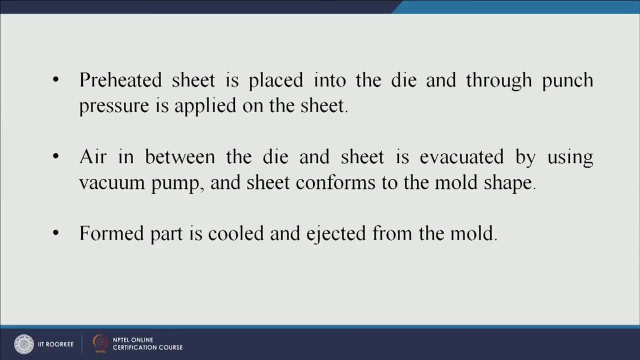 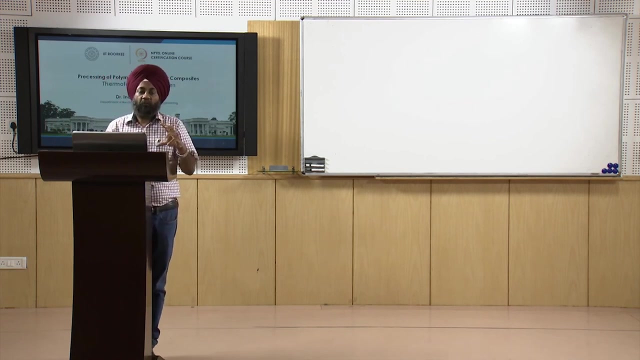 sheet is placed into the die and through punch pressure is applied onto the sheet. air in between the die and the sheet is evacuated by using vacuum pump and sheet conforms to the mold. cavity formed part is cooled and ejected from the mold. so in many cases we there can be combination of processes. also that may be if it slightly thicker sheet. we 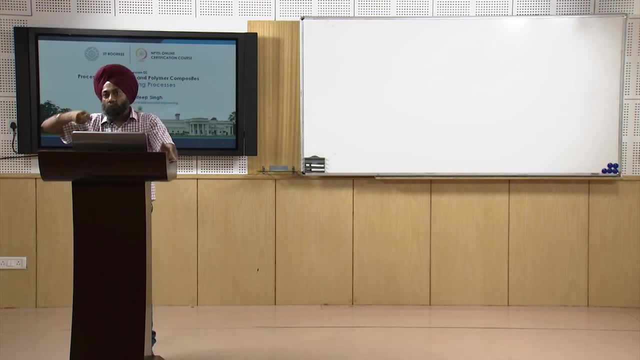 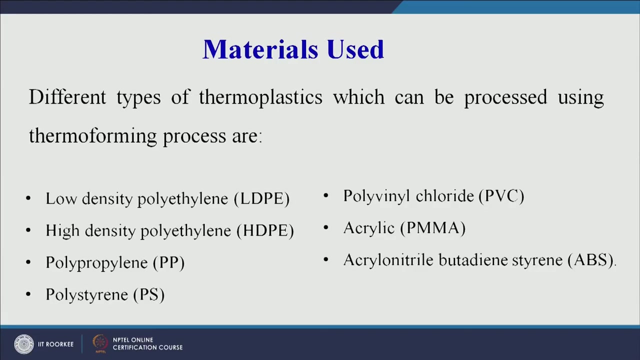 may apply pressure from both side. we can apply vacuum also, we can apply mechanical pressure also, but the basic principle will remain same: thermoforming, thermoforming, heat and forming. so the basic principle of the process remains same. now let us see what are the different types of materials used. on your screen you can see: 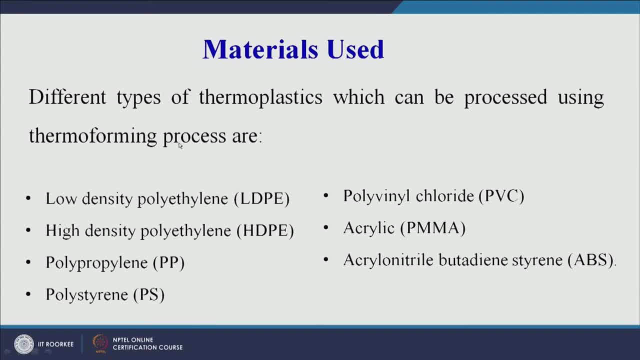 different types of thermoplastics which can be processed using thermoforming process are: low density polyethylene, ldpe. high density polyethylene, polypropylene, polystyrene, polyvinylchloride, acrylic, acronitrile butadiene, styrene. so i have just read the things for you so that 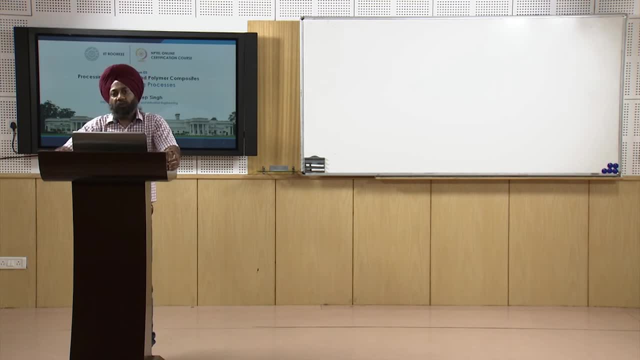 even if it is not clear on screen. you can just remember two or three or four names of thermoplastics which can be easily processed by the thermoforming process. but the major constraint is on the thickness of the sheet that we are thermoforming. if we use a very thick sheet, it will become difficult. 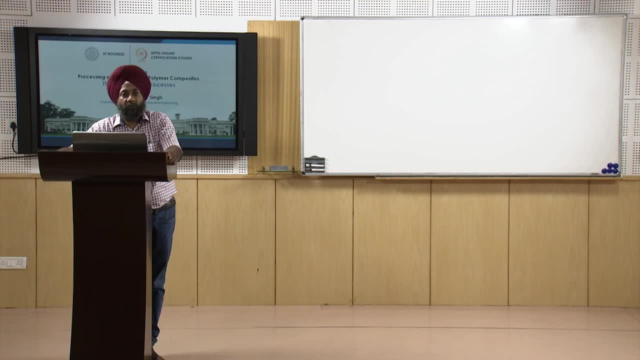 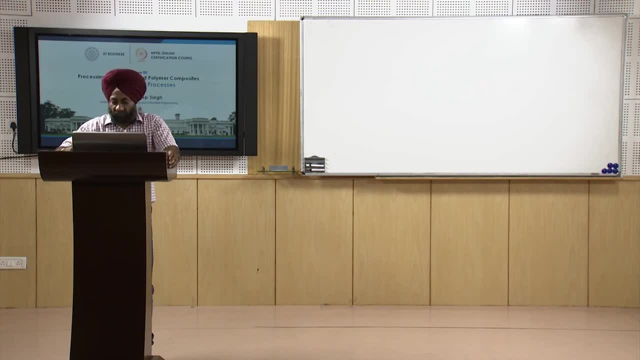 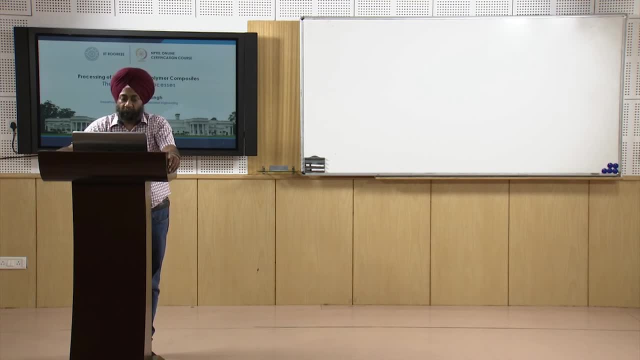 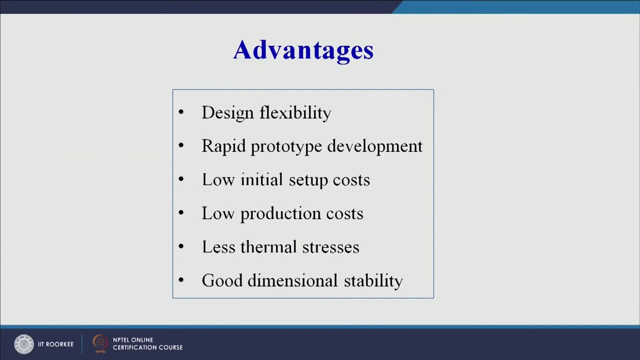 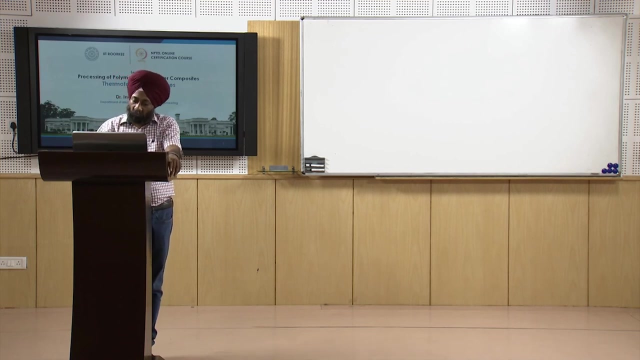 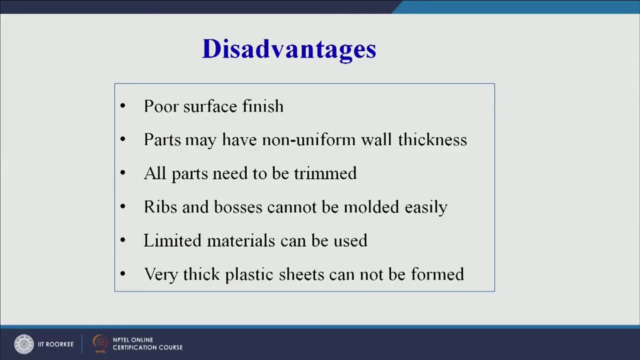 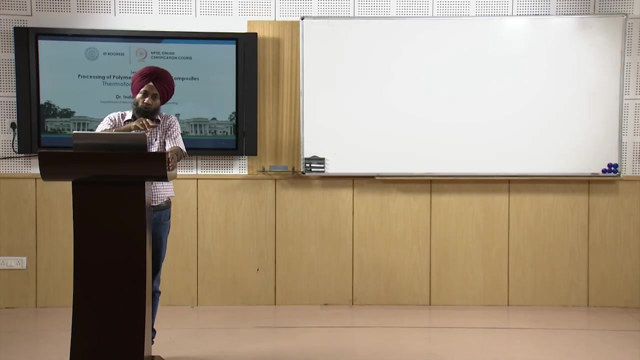 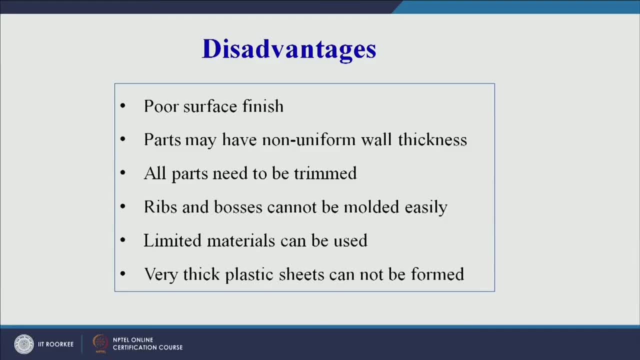 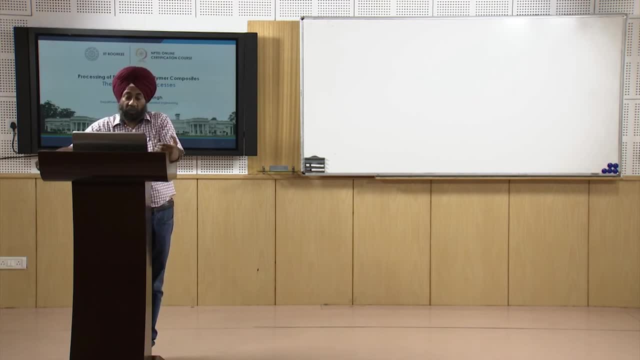 using the thermo forming process very thick plastic sheets cannot be formed, which i have already explained that it is difficult to deform the thin plastic sheets. use the thick plastic sheets- sorry, a very thick plastic sheets difficult to deform using the standard methods that we have seen today, that is, vacuum based forming or pressure forming or mesh. 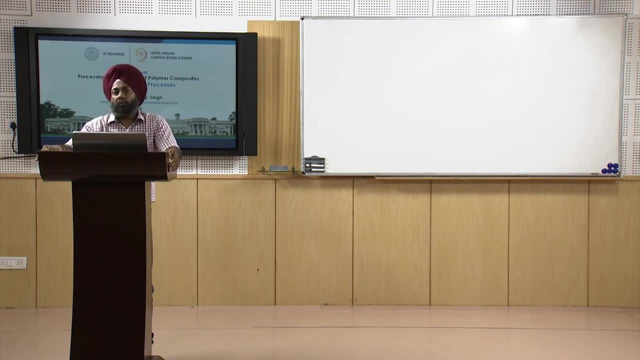 die forming. if the thickness is reasonable, then only we are able to deform it using these standard methods of thermo forming. now, what are the various application areas? so see in the process is simple, easy to operate, not very costly. so they, because of these advantages, the number of industries, are making use of this process. now, what are these application? 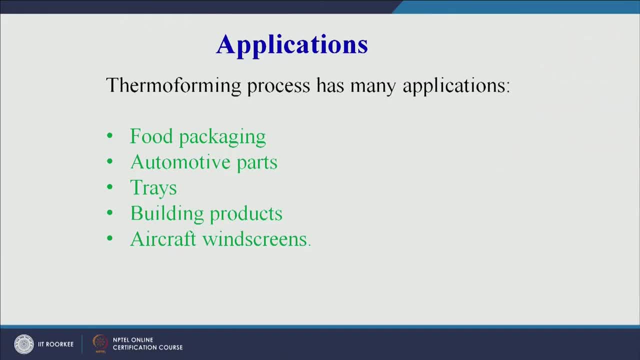 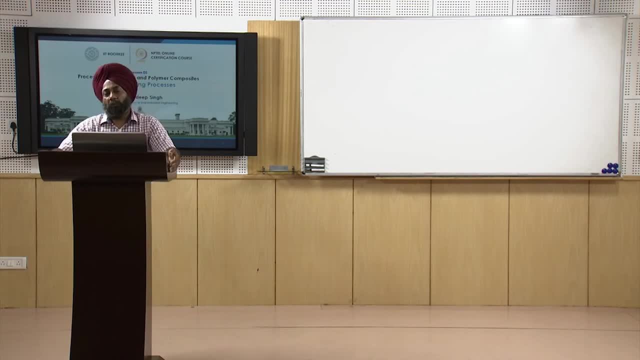 areas. food packaging is one: automotive parts, trays, building products, aircraft, windscreens, and there can be numerous other products that are made by the thermo forming process. we have tried to compile from internet two or three images that give us a glimpse of the products that can be made by thermo forming process. on your screen you can see food packaging. 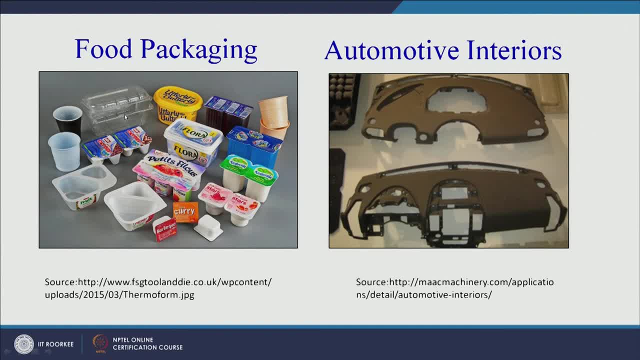 parts all of us may have used may be. this can be a strawberry box. we have used this box number of time. these type of disposable cups also have been used. disposable boxes can easily be made using the thermo forming process. even this glasses can be made, so you 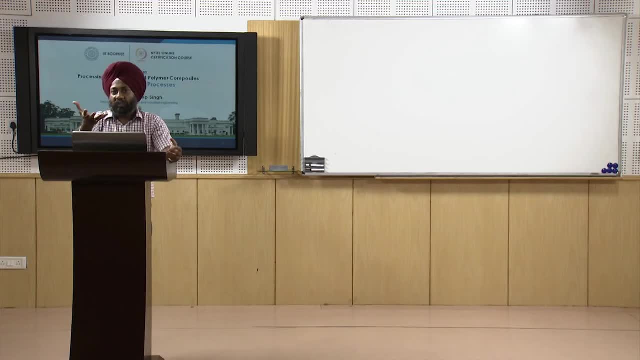 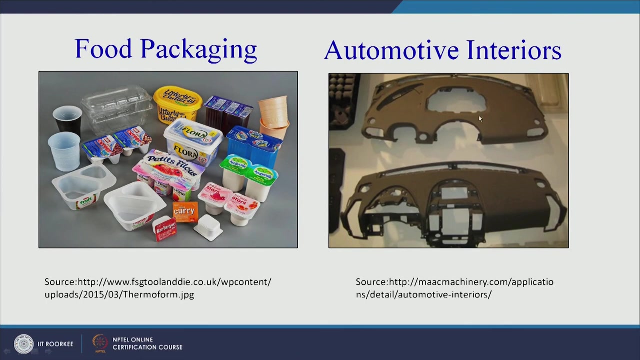 can see. you need to only have a thermo plastic sheet and a mold conforming to the shape of the product, and you can deform it by applying heat as well as pressure. on your right hand side- right hand side of the diagram, automotive interiors- you can see these are the parts that can can be easily made. 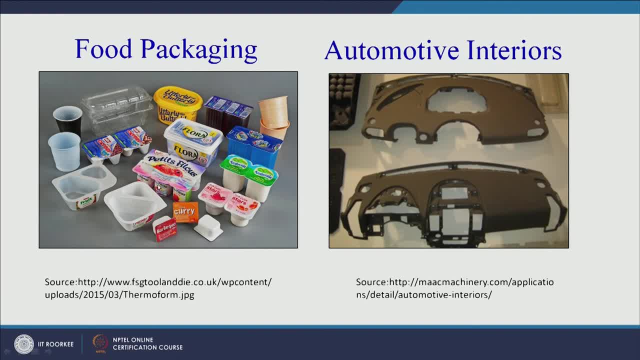 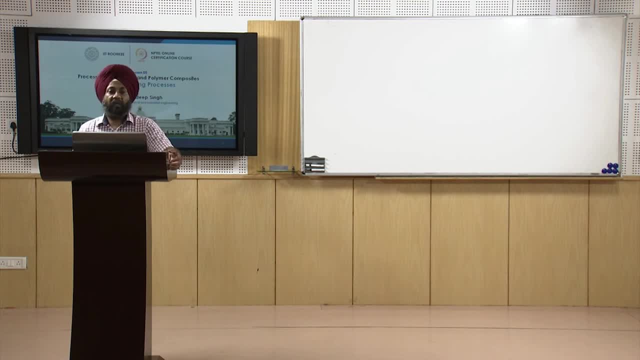 by the thermo forming process. so here we have fmcg or may be ah, household equipment or household ah products. here we have industrial scale products. so that means that thermo forming, thermoforming has got a wide range of applicability. it can be used for household products also. 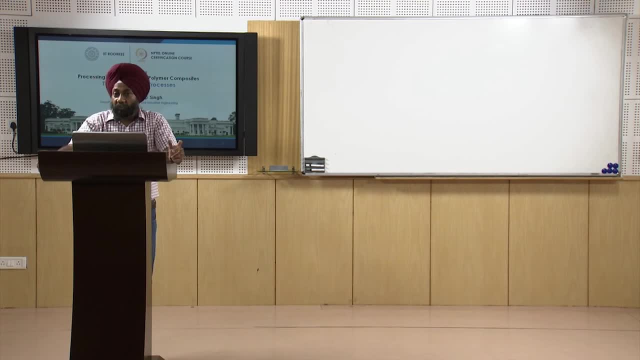 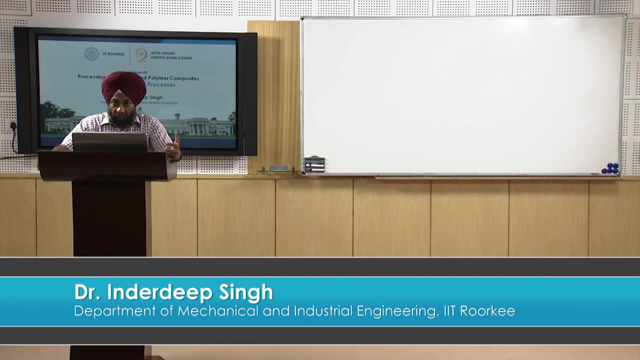 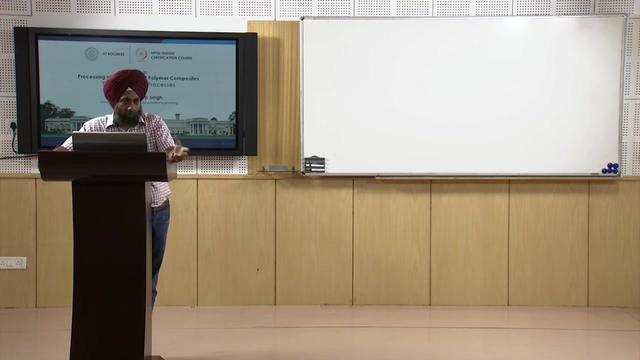 it can be used for industrial scale products also. so it is always, you can say, better to have information about all these processes which are used for making products that we see in our day to day life. now i believe that if you look at a particular product which 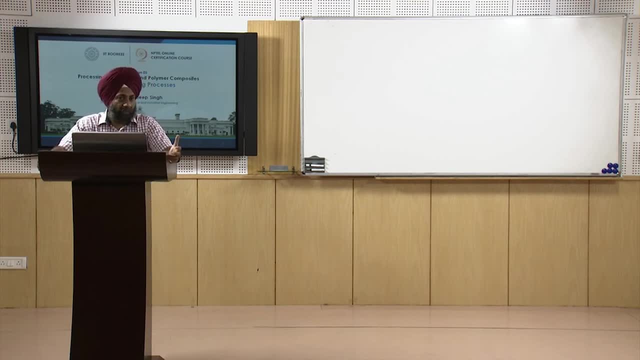 is made out of a polymer very easily, you will be able to tell that this may have been made by using the thermo forming process. maybe you may not be able to tell that which type of thermo forming process may have been used to make this product, that is, whether it is.